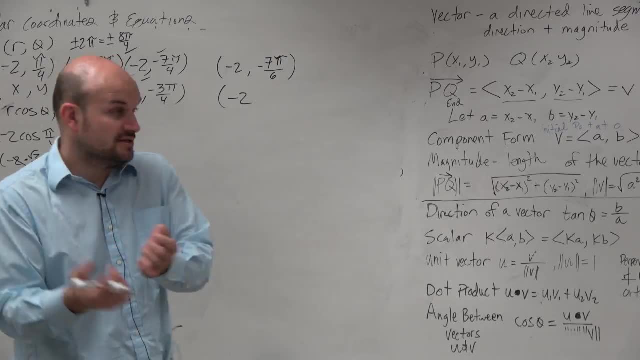 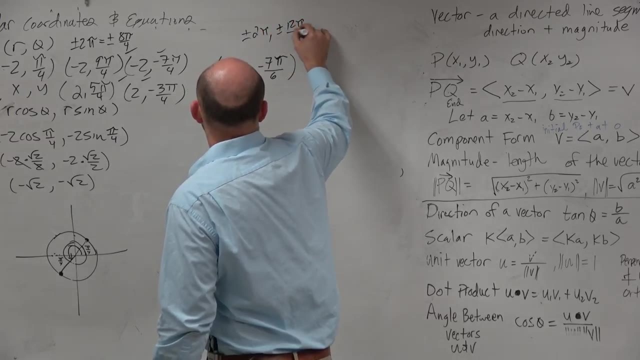 exactly the same. or a polar point? that's exactly the same. yes, So if I'm just adding or subtracting 2 pi in terms of 6, that's really adding and subtracting 12 pi over 6, right? So I'm just. 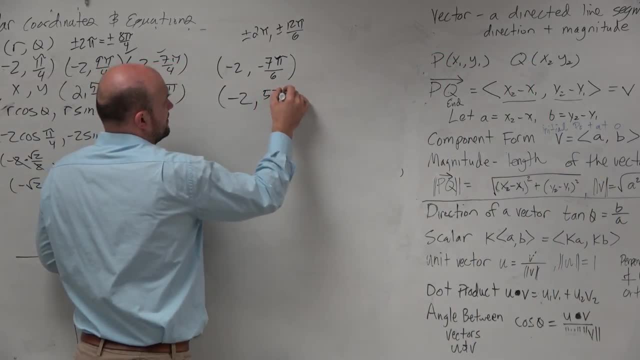 going to do this in my head real quick. If I added 12 pi over 6, I'd be left with 5 pi over 6.. If I subtracted 12 pi over 6, I'd be left with negative 19 pi over 6.. 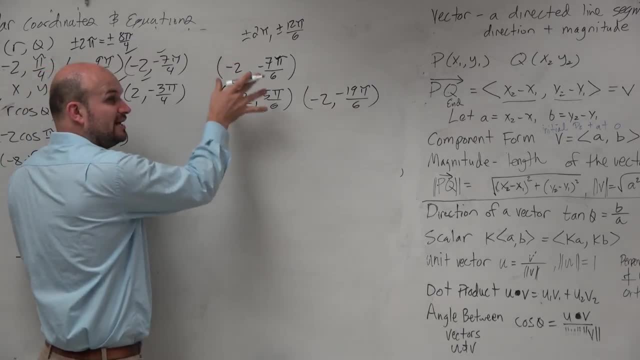 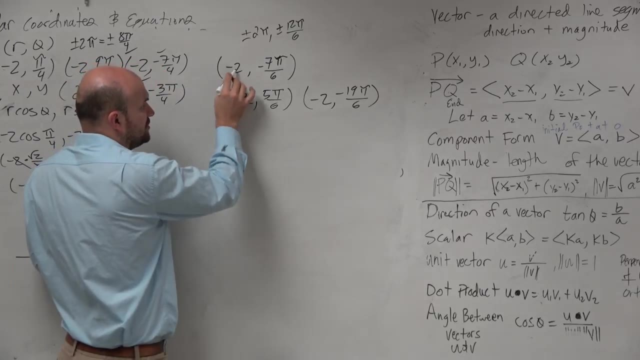 Yes, Quick, easy. Now, if I want to graph this, I explained last time why that reflection works because, again, when you multiply this negative, remember guys, this 2, this is like a negative 2 outside of cosine negative. 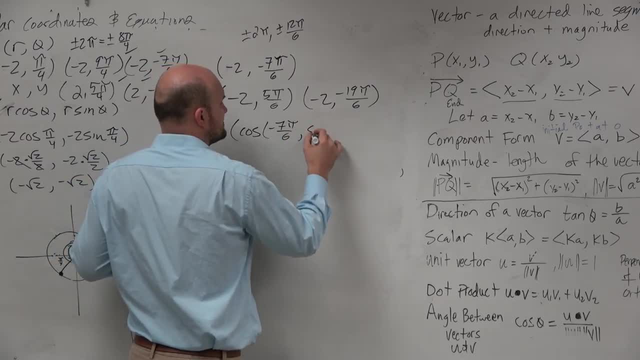 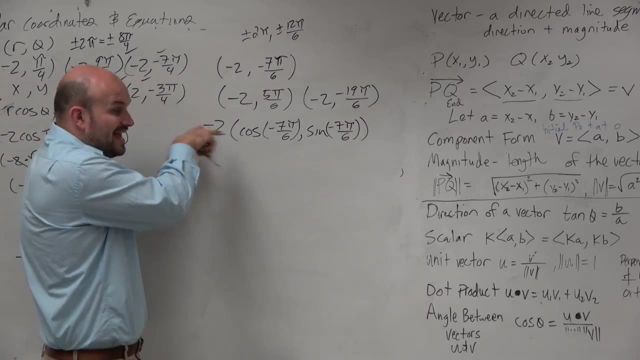 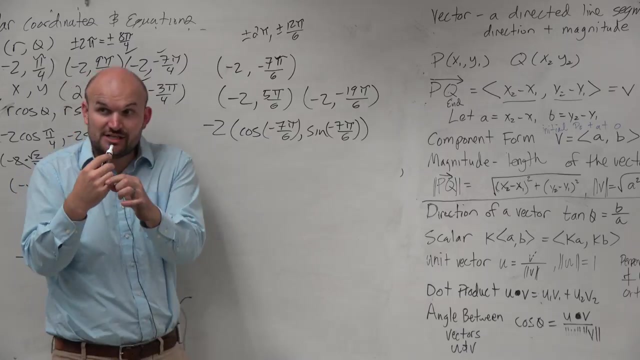 Negative 7 pi over 6, comma sine of negative 7 pi over 6.. So what's happening is, when you have the radius as negative, the radius is not changing, but that negative is changing the direction. It's not just changing the direction of the x-coordinate, it's changing. 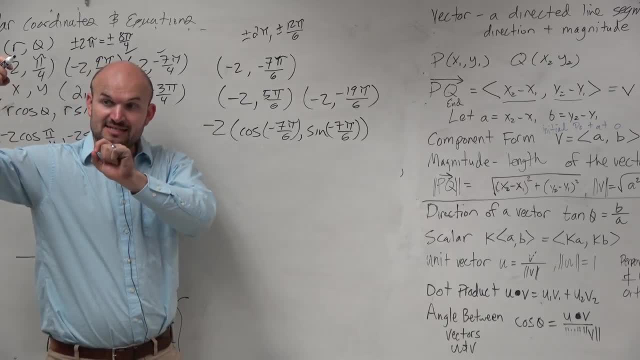 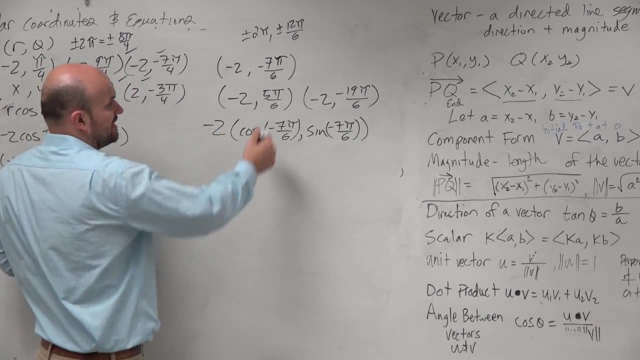 the direction of the y-coordinate, which is basically represented as a reflection about the origin. So you could sketch this, find it and therefore you can confirm it. Or another way is if you guys just forget about the negative for a second. just graph 2, negative. 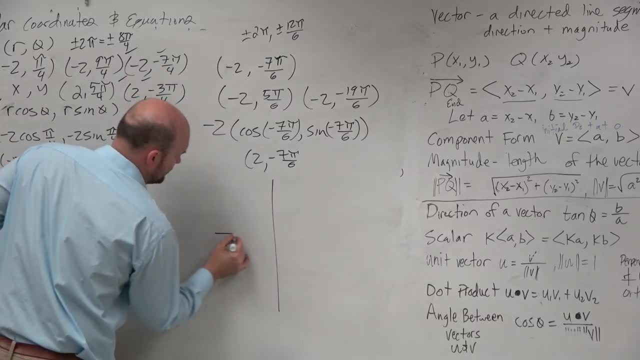 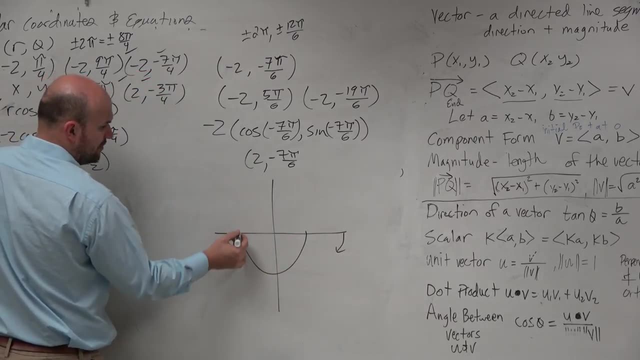 7 pi over 6.. So if I graph that angle, negative 7, so it's negative direction. Here's 6 pi over 6,. so if I go one more I'm at 7 pi over 6, right? So again, that's a reference angle of pi over 6.. 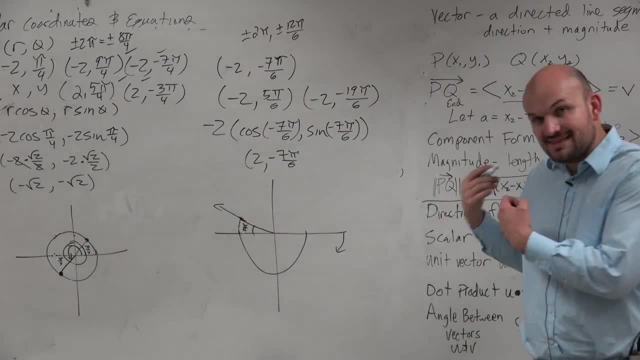 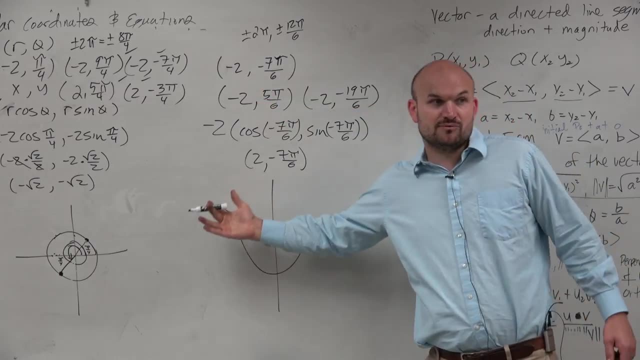 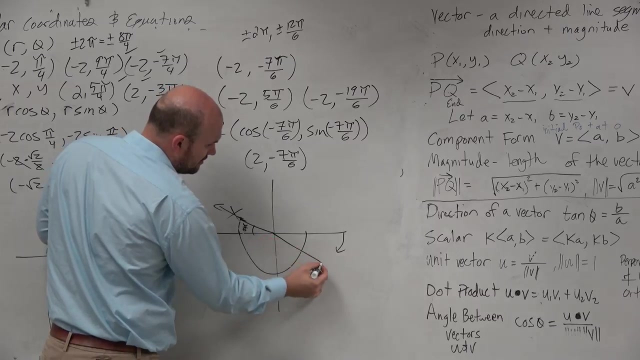 I'm pi over 6 away from my x-axis, But then think about it, guys. This is a negative, Our problem is a negative. That basically means this angle is being reflected about the x and the y-axis. So really my answer is not this one, but my point, which. 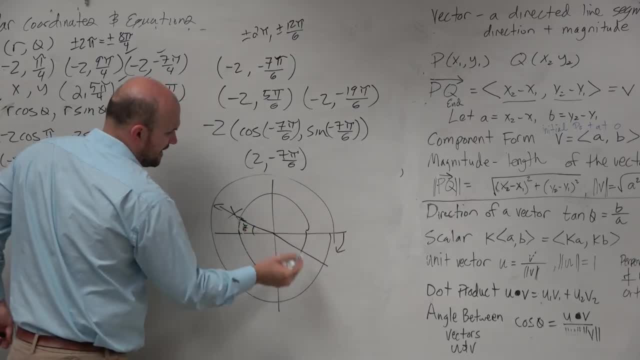 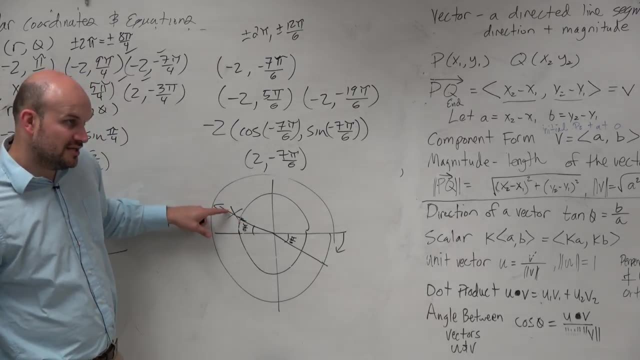 is a radius 2,. right is going to be down here. It's still going to have a reference angle of pi over 6, but it's basically going to be a reflection about the origin of this original angle. right, That's what the negative does. So now you have the point.